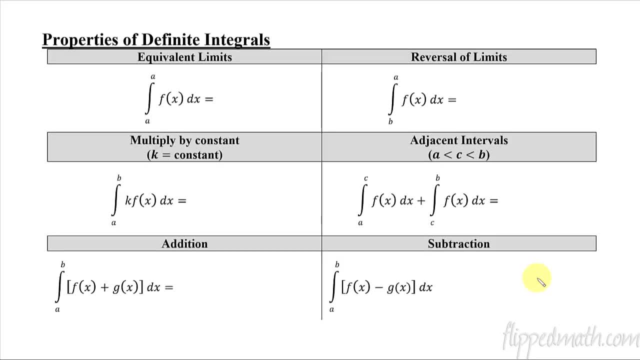 negative 1.. So that now leads us to some properties Here we have. this is the one we just did. There's a reversal of limits, right? So if it's b to a, it's the same thing as taking a to b. 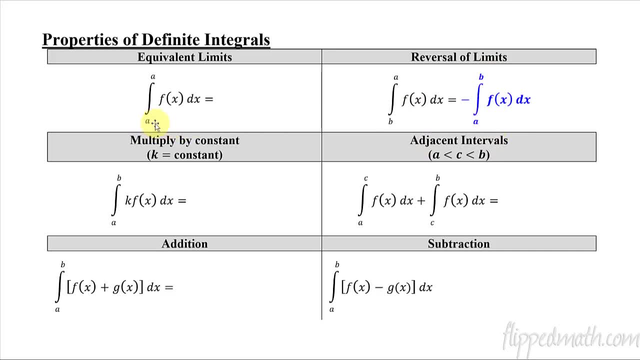 but negative. So that's the one we just did. Now what if we had an equivalent limit? So if the lower limit and the upper limit are exactly the same thing, that's just 0. You don't have anything. If your width of your area is nothing, then your area is also. 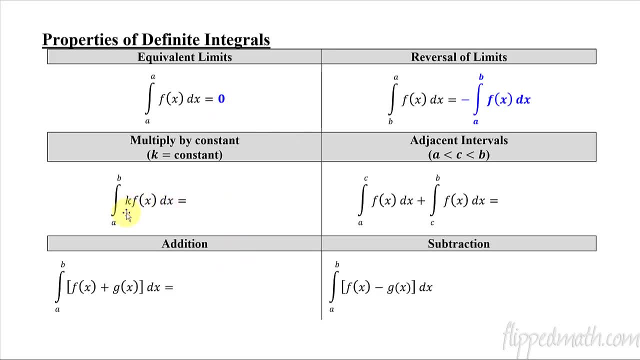 does it mean it's 0? If your width is 0.. Uh, this one multiplying by a constant. if we have a function and you have this number that you're multiplying it by, if you could factor it out. what's nice about this is it just comes to the front. 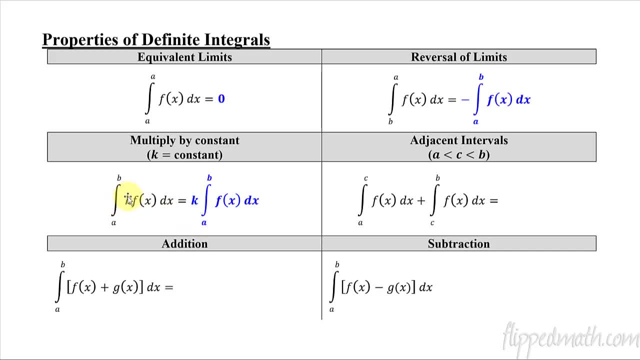 It's kind of like the constant rule with derivatives. It's just the number can just be brought to the front of it, And that's what happens here. The number can be brought to the front of the integral, and it's the same thing. This is one that's fairly intuitive. that would 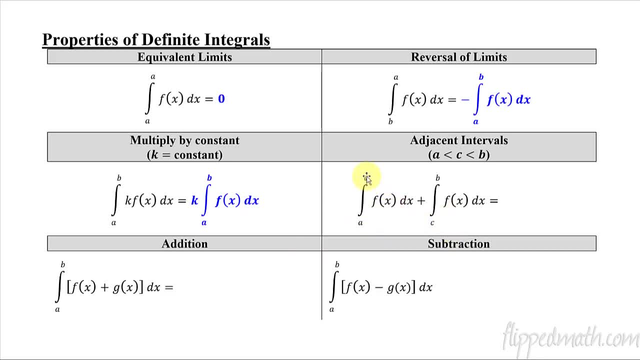 make sense to you If you're going from a to c and then you're going from c to b. I know those those letters are not in order, but that's because normally we just go from a to b. So this is what you get. You get an integral from a to b If you're going, if c is in between a and. 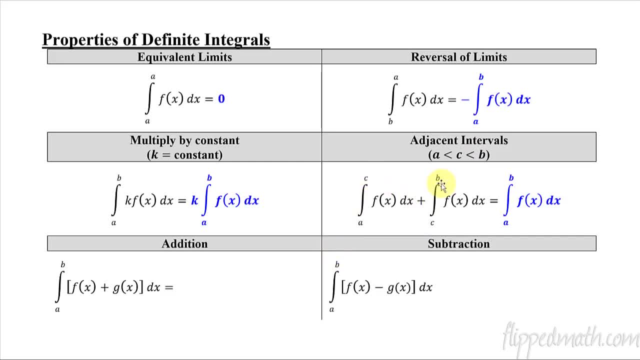 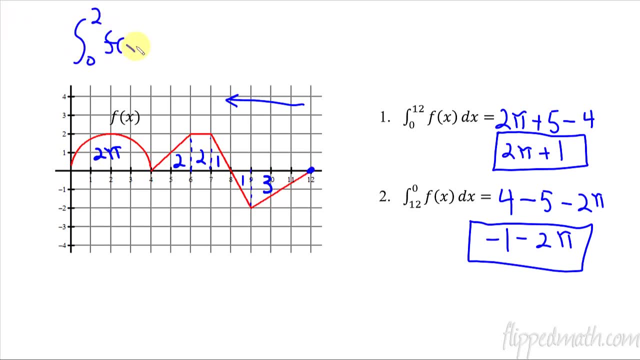 b. you're going from a to c and then c to b. Let me show you what I'm talking about with this. If I go back to this one, it's just as simple as saying the integral from 0 to 12 of f, of x. 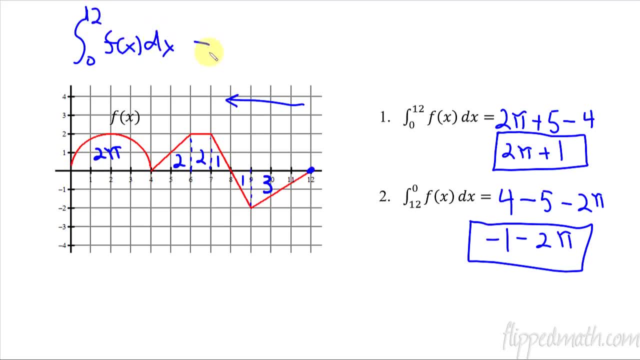 that's supposed to be 12 of f of x is equivalent to: uh, it's equivalent to saying, like I could go from 0 to 4, so I could stop here of f and then add 4 to 12 of f of x. Okay, It's pretty self-explanatory. I mean, yeah, duh, If you go from 0 to 4 and add. 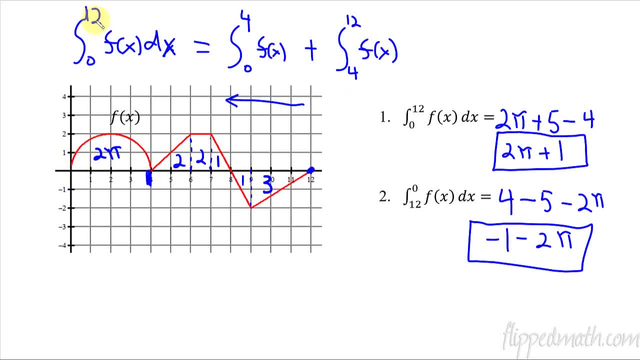 up the area and then do another area from 4 to 12, it's the same thing as just saying from 0 to 12.. But we want to make sure we explicitly state that, that we have a little rule for that. That's one. 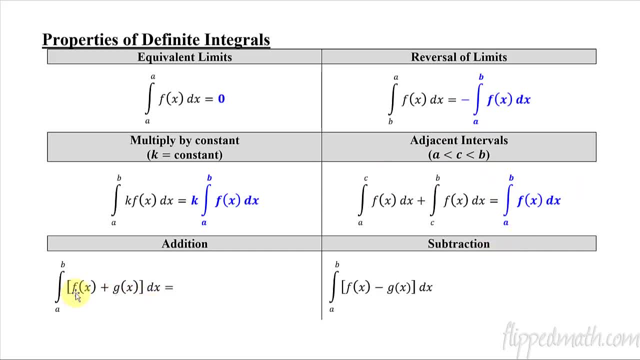 of the properties of integrals. Now, addition, real simple: You can just take these two functions separately and take each of the integrals, And that's what we're going to do. We're going to do a to b integral of f and then a to b integral of g, add them up together. So that's how you do. 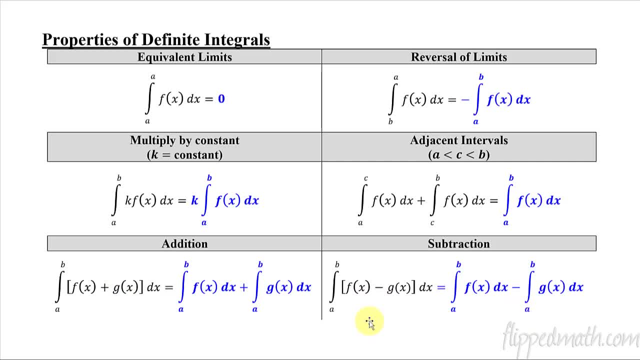 these. Uh and same thing with subtraction. Two integrals can be separated. They're the two functions I mean can be separated and take the integral of each one and add up the area under the curve. Okay, So get these properties down and now let's get into some practice and use them. 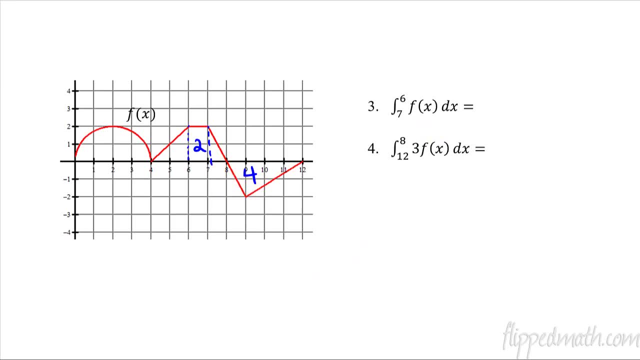 Uh, I've written down a couple areas here, cause that's what affects number three and four. And I should say this: I haven't really talked about this dx here. This dx means with respect to x, And when we say with respect to x, that's an important phrase. 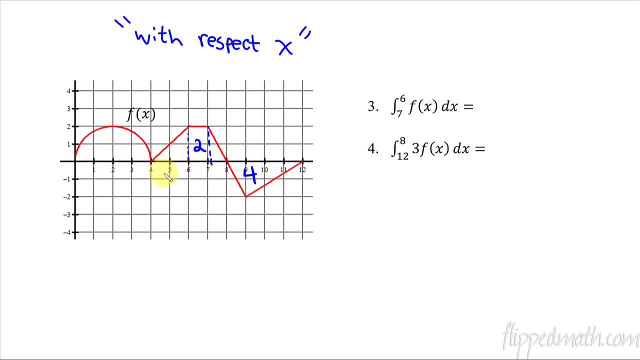 because it means we're moving along the x-axis to take the area We will later. don't stress about it yet. Well, eventually we're going to do the area with respect to y, which means we're going to do it a lot up and down the y-axis, And we're going to go this way for taking the area, like of. 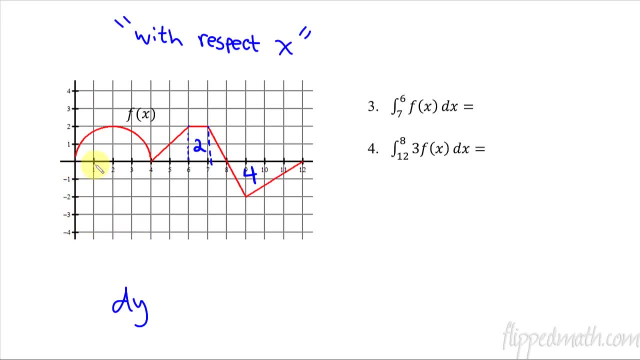 a of a curve like this. Okay, Don't stress about that yet. I just wanted to explain that. that's what the dx means. It's with respect to x, and we're going to move along the x-axis and go straight up and down for our area when we do this. All right, So seven to six, uh, seven to. 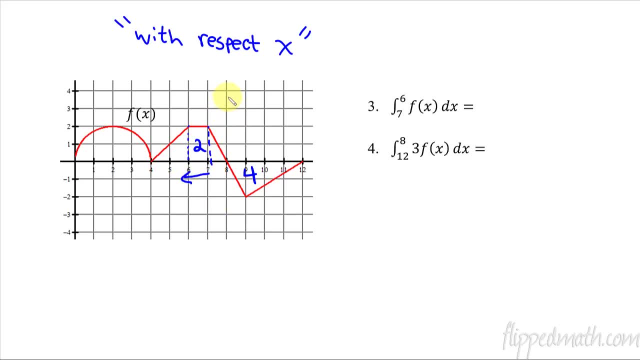 six is starting at seven and going this way: right, So you're moving left, So it's the opposite sign. So this one's negative two, and then 12 to eight, but then, oh, look at that, There's a little three right there. I almost missed that. So that's the same thing as saying: 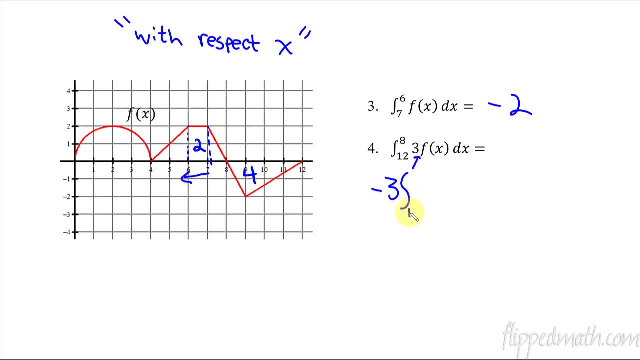 three integral. Oh, let's do this negative three integral. And then I'm going to switch the signs eight to 12 of f, of x, dx, So I can use properties to manipulate this around and change this up a little bit. So then this is going to be negative three. 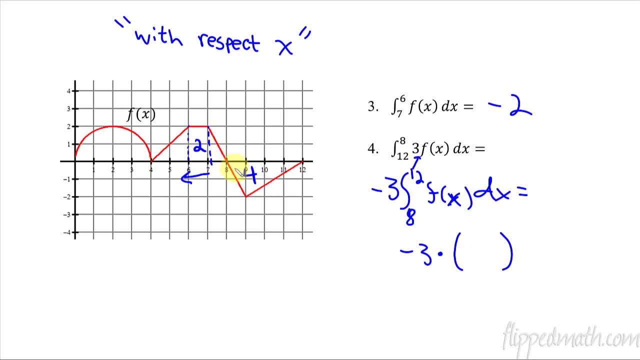 times. And then the area between eight and 12, I already figured out- was negative four, right, So that's a negative four. So then I have a equals a positive 12.. So, using properties of integrals, there's a few different ways that you can manipulate these expressions. 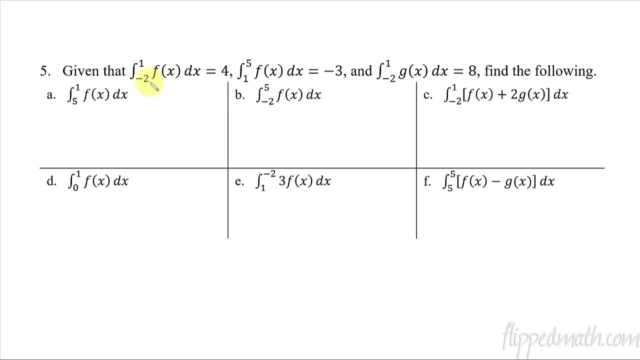 to come up with your answer. Okay, Using them some more. Now I have one, two, three different integrals: This one's f of x, this one's f of x, this one's g of x. So be careful there. 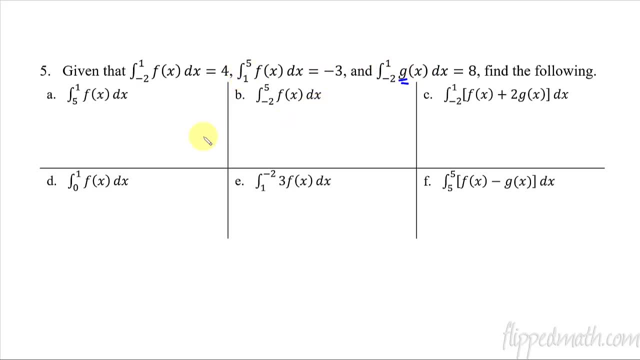 And then you just have your negative two to one, your different boundaries on your lower and upper limit. So what we're doing for this first one is we're trying to figure out from five to one of f, of x. Well, what we do know, 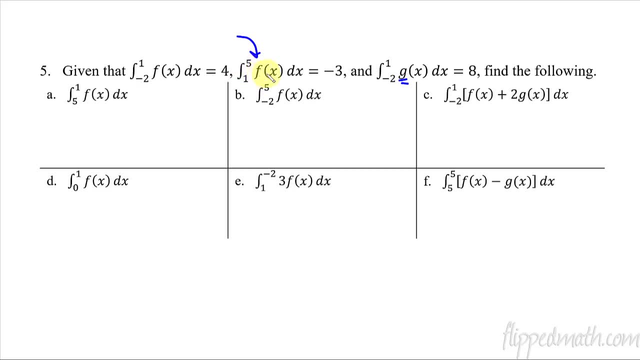 is right there. we know that from one to five the integral of f of x is negative three. So if I'm just switching the upper and lower limit, that becomes the opposite and is positive three instead of negative three. negative two to five. 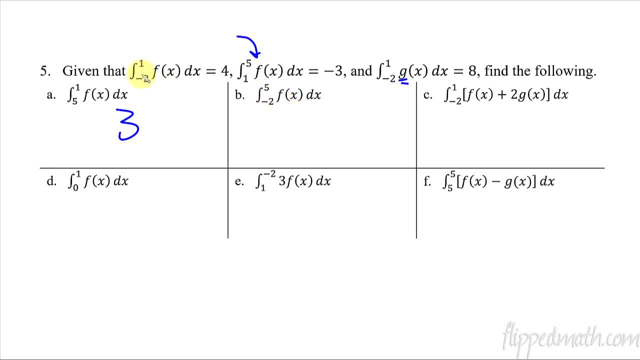 So, of f, I don't have negative two to five, but I have negative two to one, and then I have one to five. This is basically this. here, It's these two integrals that are being added up. That's what this one is, So then I have to just figure out. okay, well, that's a four plus a negative. 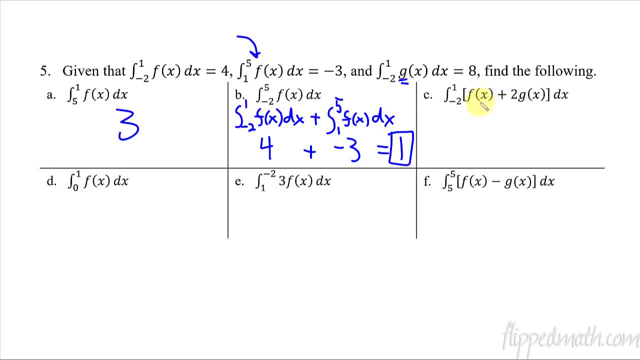 three, So that equals one, And then this one: here I'm doing negative two to one of f of x. So this addition means I can separate them and take them individually. So the negative two to one of f of x, that's a four here. So I'm going to say four plus, and now I'm 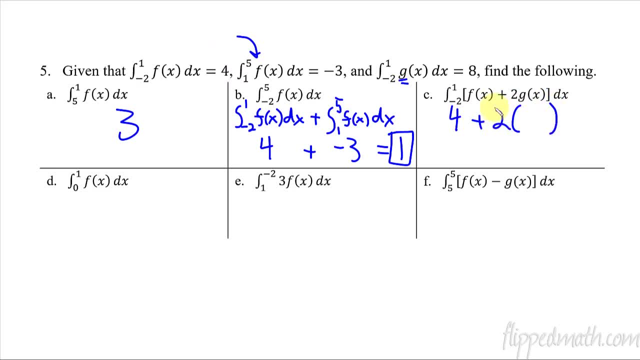 going to do two times. What is the integral of g of x? from negative two to one, That's eight. So we just have four plus 16 gives us 20.. Here's an interesting one: Zero to one of f of x. Well, I have negative two to one, So zero to one is inside this integral somewhere. 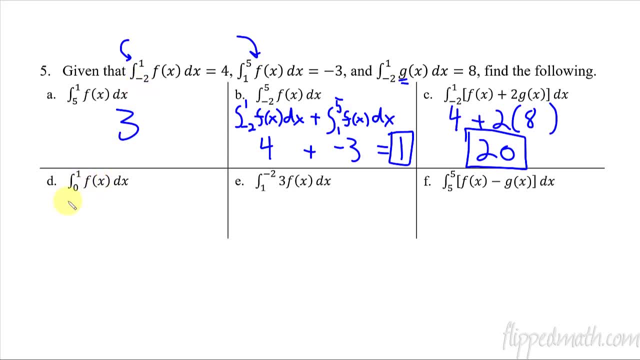 but I don't know exactly what's going on from zero to one, So this is one that you cannot figure it out, So I'm just going to write down: cannot be determined, And sometimes that'll be one of the multiple choice answers that they'll give you on an AP exam that you 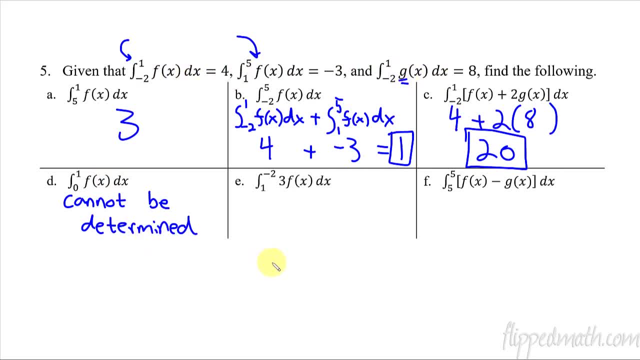 can't figure it out based on the information that's given. You need more information to be able to do this one, So I'm going to go from one to negative two. That's flipping these again. right, And it's f? Yes, it is, So I'm going to flip these back. pull the three out. This is similar to another. 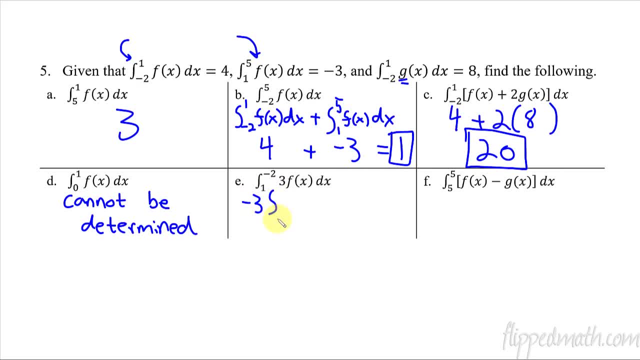 one. I've done. So pull the three out and make it negative, and then go from negative two to one of f, of x with respect to x, So then this is negative three times four. All right, So that equals negative 12.. 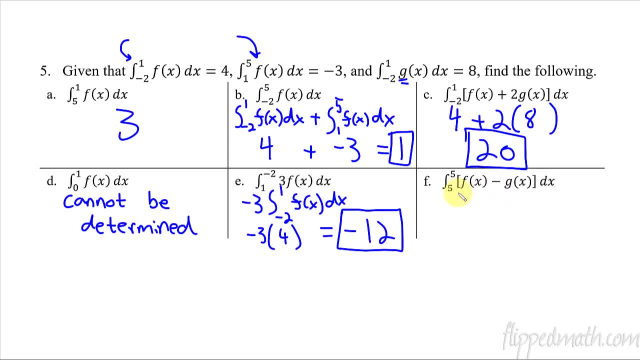 And in this one I have two functions being subtracted, but my lower limit and my upper limit are identical, So my width is zero. There's no area here, So we just have nothing for our area. And now some piecewise functions. Don't worry, this is not going to be that. 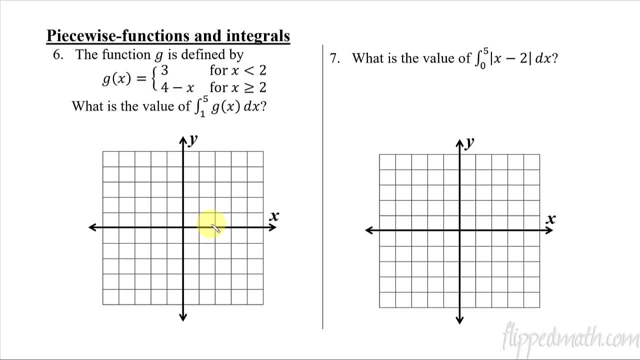 difficult. Sometimes we get scared of piecewise functions, but it's really not bad, So we just need to. well, if you don't know how to draw piecewise functions, then yes, this is challenging. Sorry, But uh, let's do this. line y equals three. Oh, that was so close. 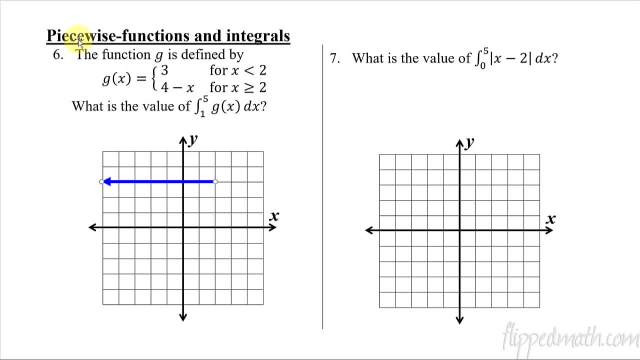 to being straight. Oh, that was awful, I cheated, I used a drawing tool, Okay, So then we have a line: Uh, we have: y equals three when x is less than two. Let me put an open circle here, So open. 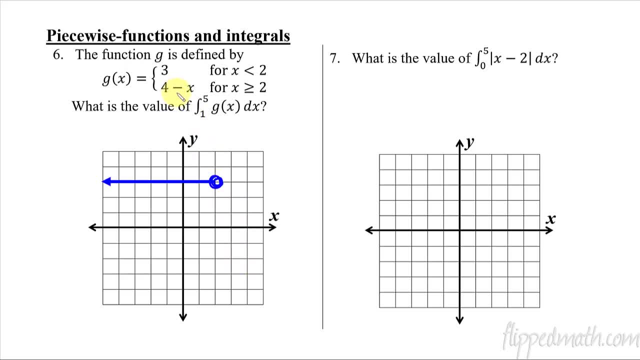 circle right there at two and then four minus x. So that would be a line that would have a y intercept of four, one, two, three, four and slope of negative one going down like this, And then it's a solid circle there And then it's going to keep going down. that. 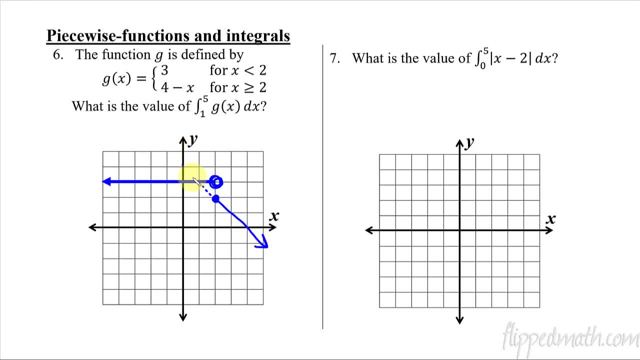 way. Okay, And then let me erase this part that I didn't need. All right, There's my piecewise function. So now I have this piecewise function. I'm doing the area under the curve From one to five. So I'll start here at one and I'm going up until I get to five. So the 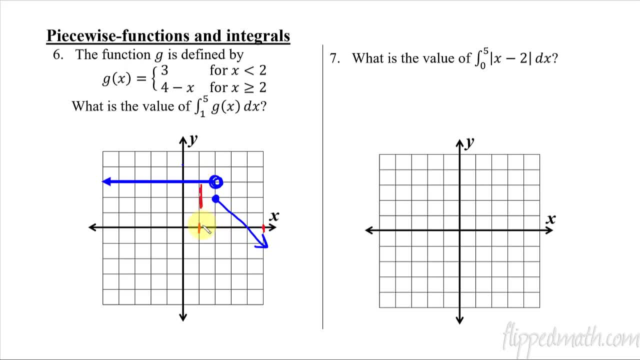 area under the curve. this is weird, because you have this area here, but then it jumps. Well, it doesn't matter, We're still going to just have this area right there. And then, even though it jumps, it just jumps down and stays between the function and the X- X axis. 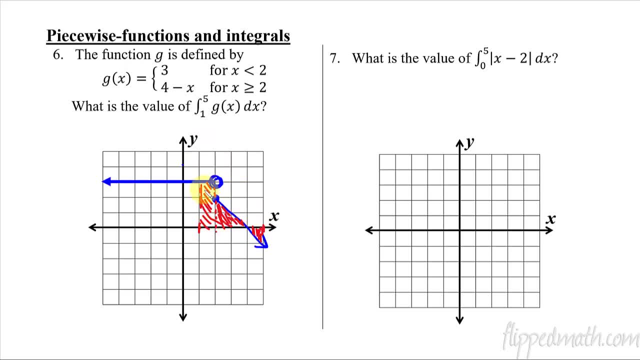 And then again here. this is now negative area there. So what I do is I just take each of these pieces. even though they're weird shapes, it's still nice geometric shapes for us. So this rectangle here is a three, So I'm going to say three And then I add this triangle. 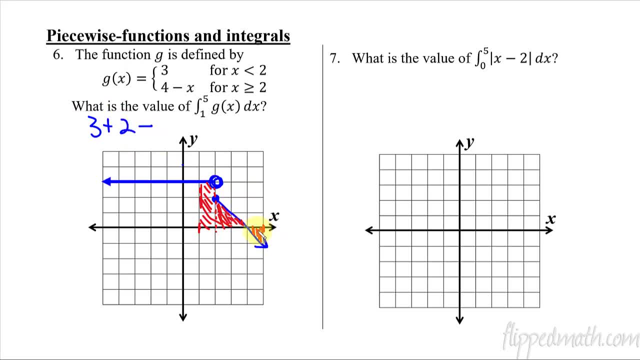 is going to be two. And then I subtract the area of this little piece here which is just a half, So I have five minus a half, So that equals four and a half or 4.5.. So the big point of this is, when you have piecewise functions, you still treat it just the same, If you can. 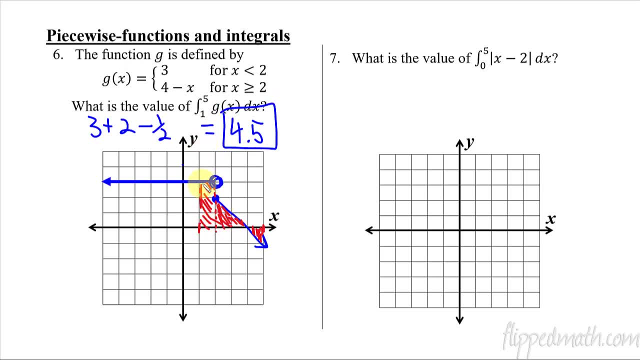 think of it geometrically, the shape of it. what it's doing is it's the function, and then right underneath it to the X axis, And then, even if it has a jump, that's okay. You just don't include this piece. 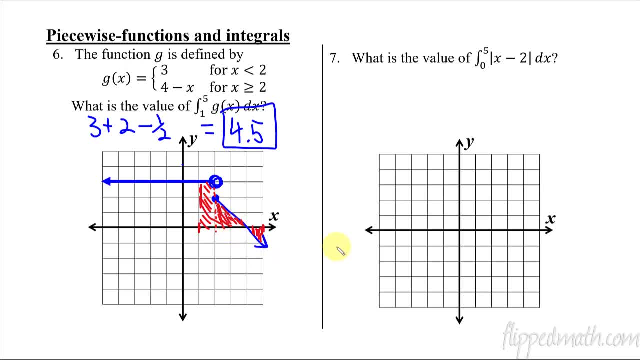 Here you just jump to where the graph is and then to the X axis. That's the area, the boundaries of the area. All right, here we have an absolute value. I want to mention this one because, well, a couple of things about absolute value, but these really are piecewise functions. 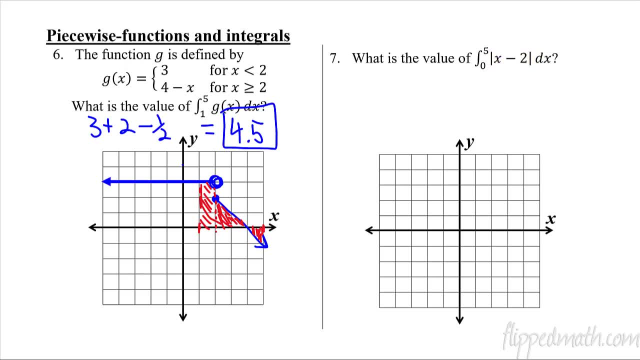 What is a? what is an absolute value graph? look like It creates a V shape, So you should have a graph like this. It's got the V right there at X equals two, shifted right Two, And now we're going from zero to five. So I'm going to take this area here and then. 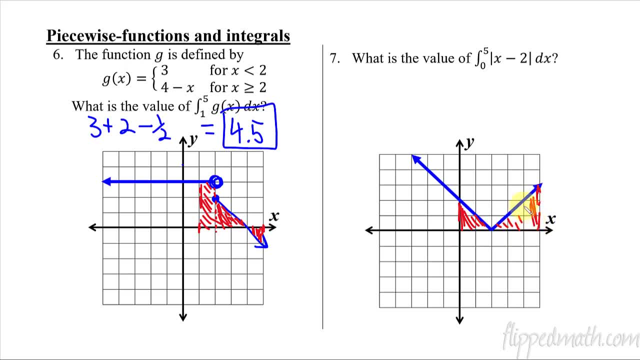 this area here all the way up until I get to five. So that's the area, So the. this is what this integral represents. So when you can think of absolute value graphs, think of them as piecewise functions, and then it's a lot easier. 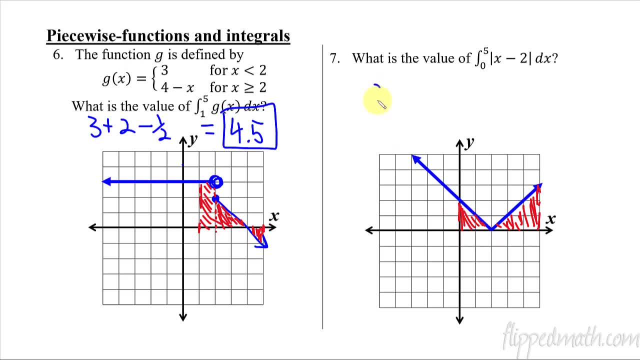 to figure out. So what is this here? This is the area of two, So I'm going to say two And then I add, because this is all above the X axis, That one is half of nine, right, Yes, Nine, So 4.5, half a nine is 4.5. And that equals 6.5 for my area under the curve. 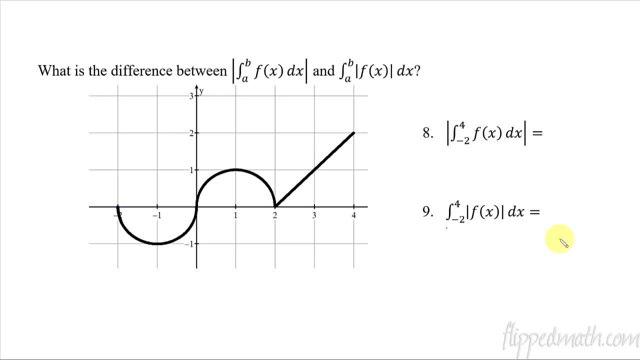 of this absolute value function. Okay, Two more things. The first thing that we need to find out is how to put this in the right order. So let's say we want to put this in the right, to talk about the difference between these two things, these absolute values. 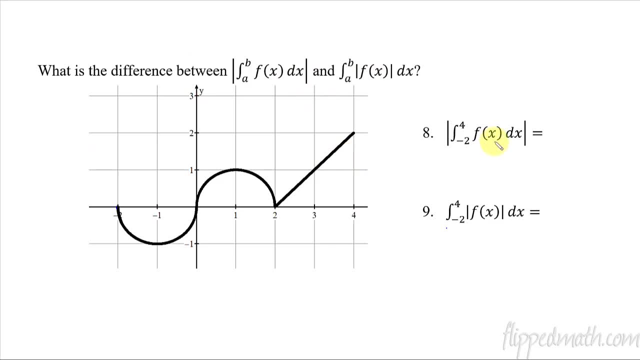 these are not identical. they have different answers. so let me show you first of all, when you have the absolute value on the outside of the integral, all this means is you figure out what the integral is and then you take the absolute value of it. so I'm gonna have the absolute value of. so what is this? 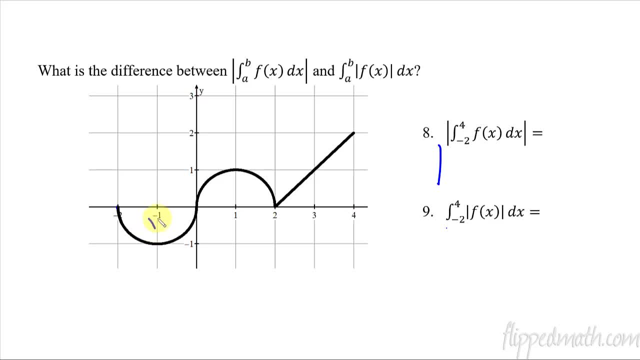 this is. this area is half a circle, so it's pi over 2. the radius is just 1, this one's pi over 2 and this one is 2 for that area there. all right, so I'm going from negative 2 to 4. this is negative area, so I'm gonna say negative: pi over 2. 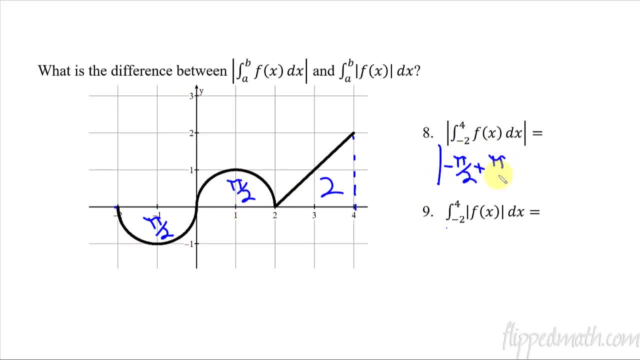 this is positive area, so I'm going to add pi over 2, and then the last area is also positive, so I will add 2, and then that equals is those cancel to 0, you get the absolute value of 2, which is 2. so there we go for that one. now, this one's. 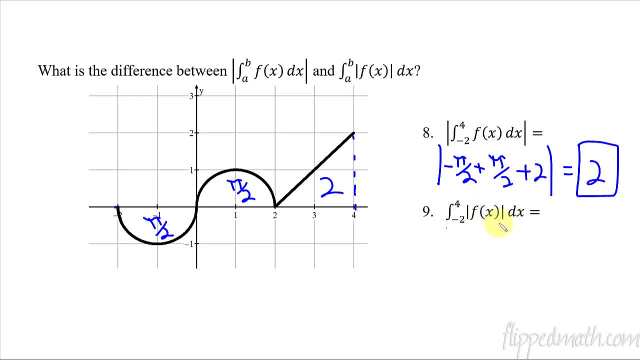 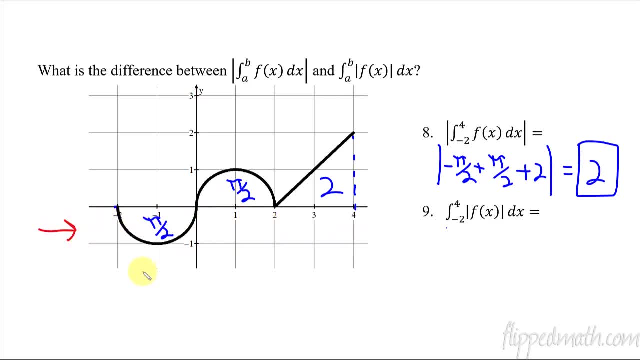 underneath the x-axis down here. anything down here will go, will flip up here to the positive side. so this part of it would be: oh, that was so close to drawing that. well, this would be a graph that looks like that and it's positive pi over 2 now instead of negative. this parts gone and it just jumps up here. so 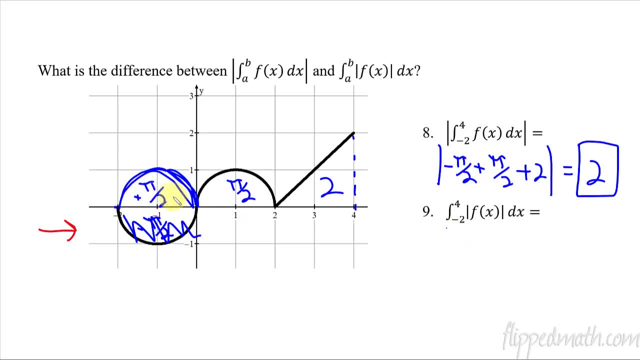 now, when we do this, this is going to say we're going to take the area of these pieces, so it's pi over 2 plus pi over 2 plus 2, and so then that equals. this simplifies to just pi. 2 halves equal a whole plus 2. so you: 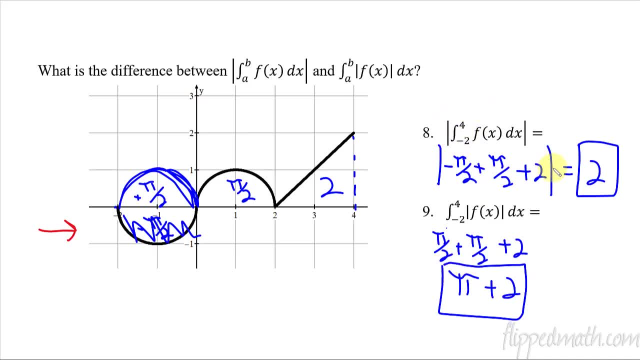 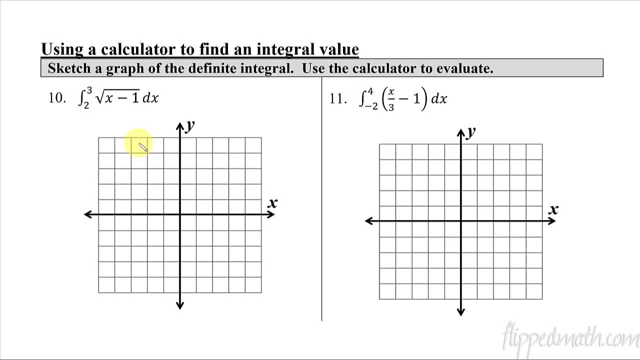 can see very different answers. 1 is taking the absolute value after you're done. one is taking the absolute value first, which makes all of the area positive. and our last thing: you need a calculator. for if you don't have a calculator, pause the video and go grab one, because you need one and you've got. 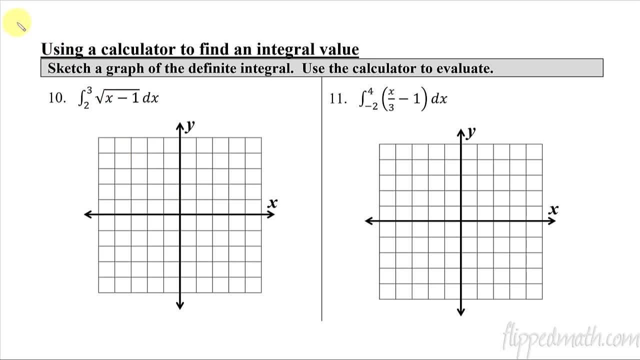 to practice. it's amazing how many times you need to practice to get it right times. kids can't do this. when I see them come up for masterchecks because they actually didn't ever practice this with a calculator. Let's start off by sketching the graph of these things. So the 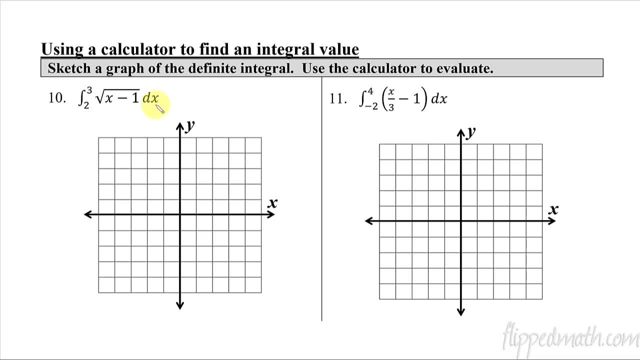 graph of this: one x minus one square root. So remember, square root graph goes something like this: It's like if you could have a parabola like that, it's the top half of the parabola. That's what this really is: square root graph. So we're going to shift right one and then we have a. 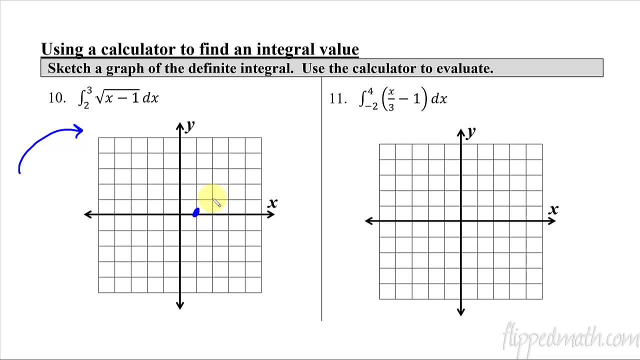 parabola that goes. let's see if I go over one up one, if I start from here and go over four, one, two, three, four up two, because that's like a square root curve. Okay, mine looks almost like a straight. 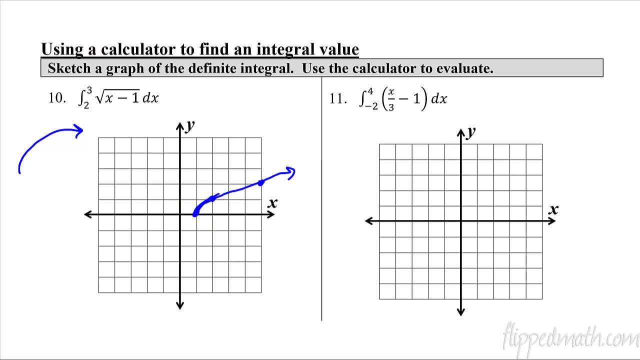 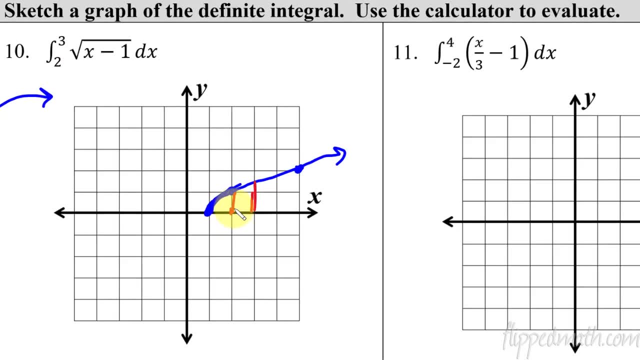 line. Sorry, it's supposed to be curved right there. All right, so square root graph. And then I'm looking at the interval from two to three. So I'm going to go from two to three. That's a really tiny area right here. That's it. This is the only part I'm looking at. So what is the area of that? 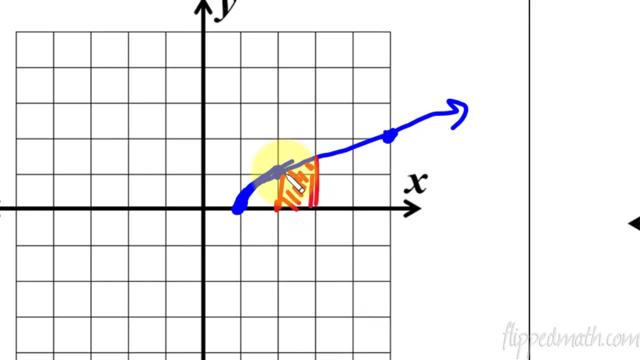 Well, you haven't learned how to do this yet. We're going to learn, but I'm going to show you how to do it. So I'm going to show you how to do it. This looks like it covers this one square, and then a little bit more, maybe a quarter more. 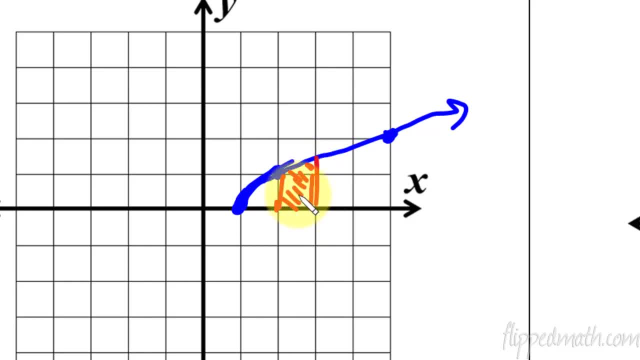 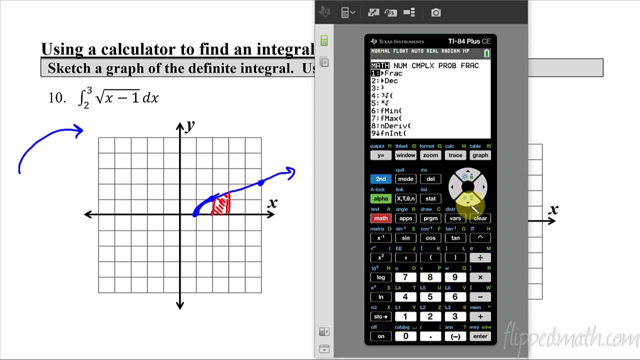 but we're not going to guess, We're going to let the calculator do this for us. So grab your calculator and here's how it works. So I'm going to type math, option number nine, So I could just hit math nine or scroll down here, And this does a functions integral. So if you don't have a TI-84,, 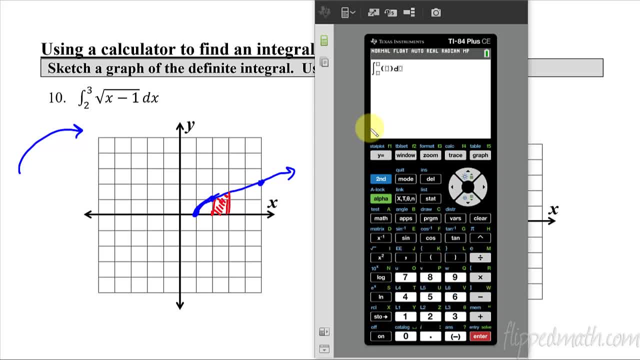 if you have something else you'll have to figure it out on yours, But so you just have to Google. how do you do an integral with a integral With a whatever Casio or HP calculator, whatever your model is. So this case I just do the lower. 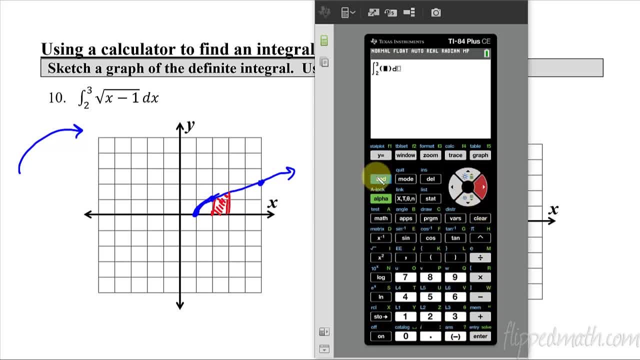 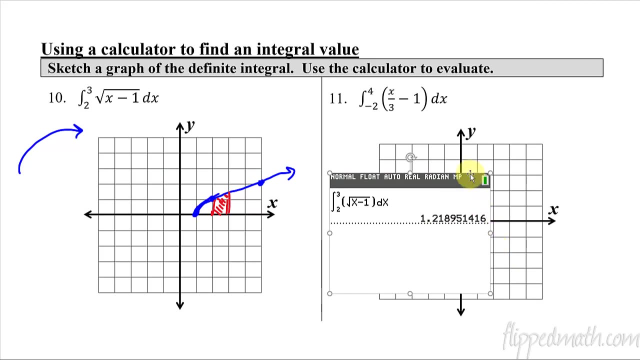 boundary is two, upper boundary is three, And then I type in the square root stuff, So square root of X minus one, And then I come out here and I'm going to do it with respect to X: Enter: Okay Yeah, Oh look, drag this over here. So that's really close to what I thought it might've been. 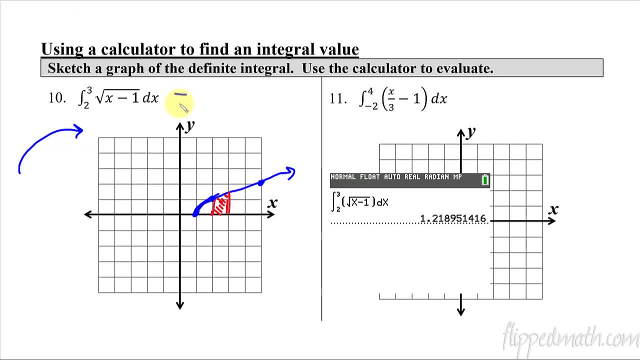 I was guessing a little bit more than one, like one and a quarter or so. So this is one I should say approximately, not equals approximately 1.21.. And then I could either go eight or I could round up to nine. I'm going to write four decimals, just so you can see it, but I could say either. 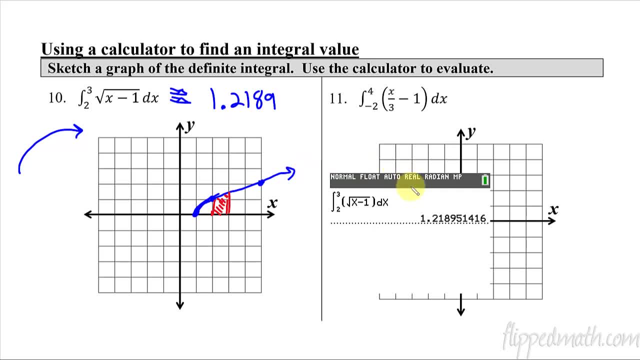 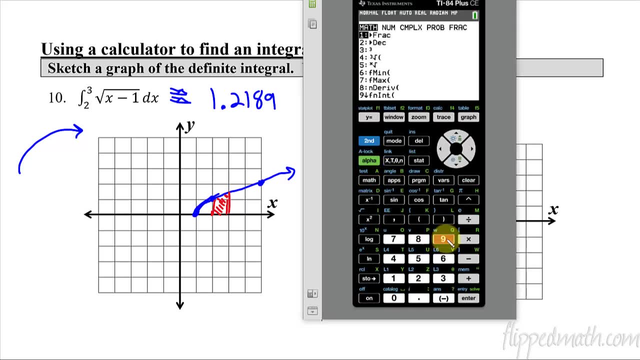 1.219 or 1.218, either way works. So let's do that again for this one. In fact, let's have you pause and do it on your own, but let me just remind you math number nine. That's how you get the. 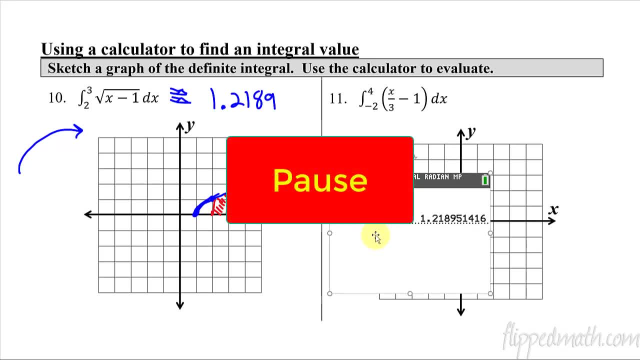 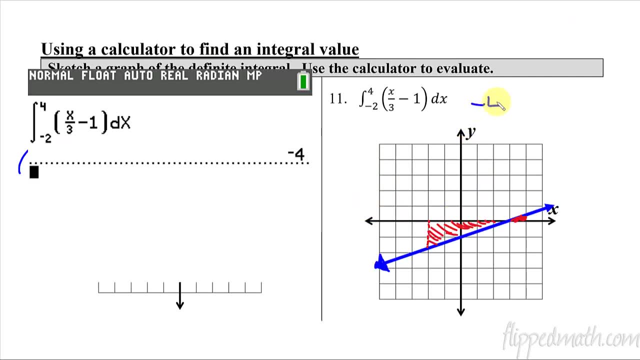 integral to show up here. Okay, So go ahead and pause this and try that one on your own, And you should have come up with negative four on the money. So this is a little bit weird because it has these shapes that you'd think you could do geometrically, but they're pretty tricky because 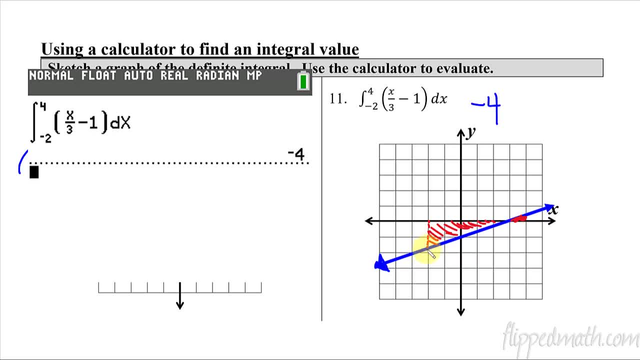 they do not end right on a nice perfect end point. See this here: from negative two all the way up to one, two, three, four, So you have this negative area and then a little bit of a positive area, And so that does throw things off a little bit for for calculating geometrically And that's. 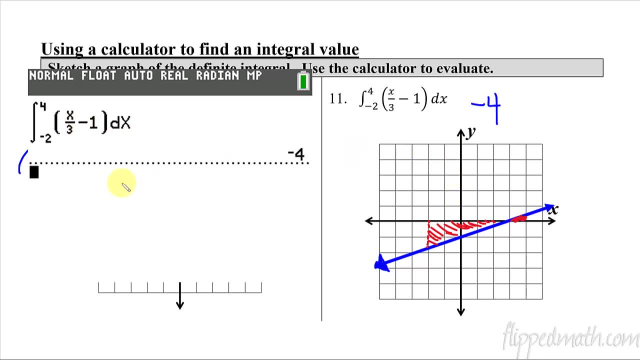 where it's nice. If you didn't know how to do it, but you're allowed to use it a calculator, then just do math nine. So again we'll. we'll learn in the next couple of lessons. We're gonna learn how to do this the long way by hand, but a calculator, if it's allowed on. 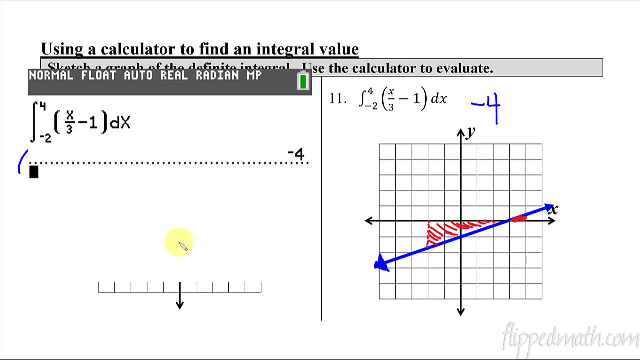 the problem. math nine: super fast and easy to calculate the area under the curve. Okay, We've covered everything for this lesson. rock that macro check and I'll see you back in the next one.